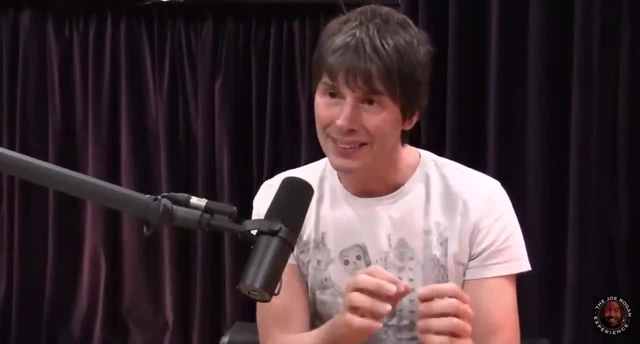 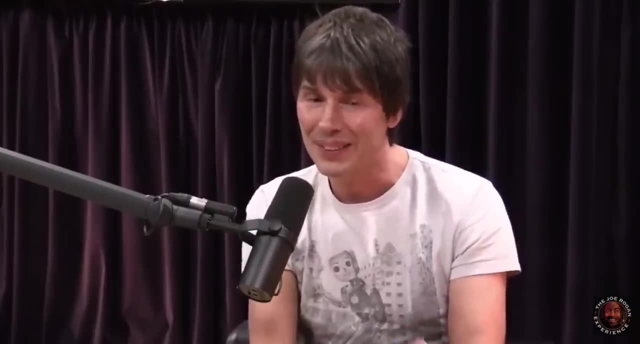 They're surrounded, this region where if you fall in it's called the event horizon And if you go across that horizon then you are going to the center. There's one way of thinking about it which is quite cool, which is that the time and space sort of flip is one way to think about it. 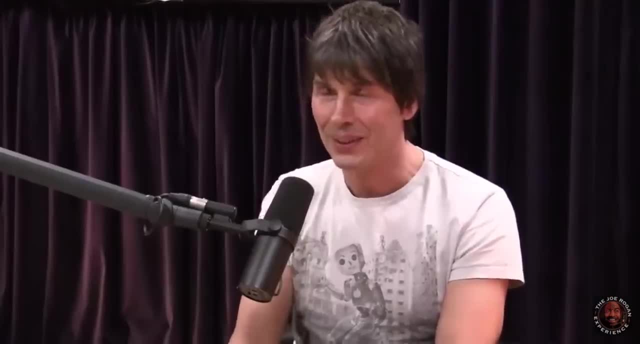 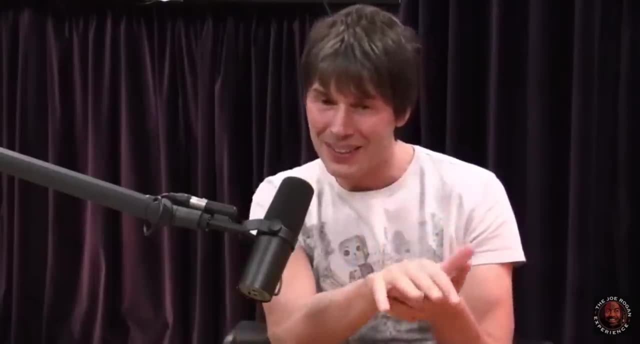 So, in the same way that we are going into the future now, So we're going to tomorrow. There's nothing we can do about it. We are going to tomorrow. In the same way. if you fall in across the event horizon of a black hole, you are going to the middle, the singularity it's called. 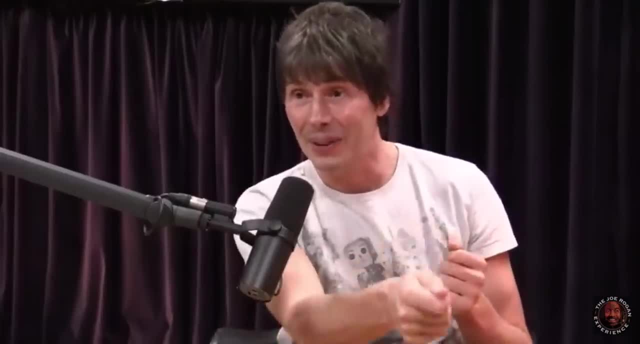 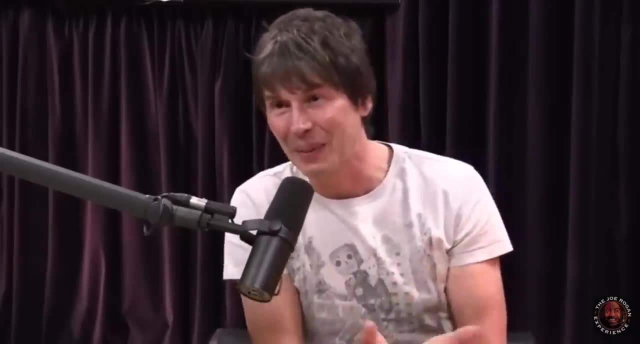 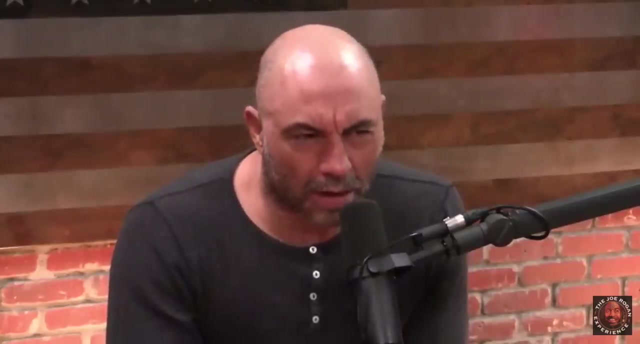 So that's your future. Every line of your future points to the center of the black hole. So it's kind of the ultimate of no escape, the ultimate prison. You're going to get squashed to an infinitely dense point. So not every star becomes a black hole at the end of its life. 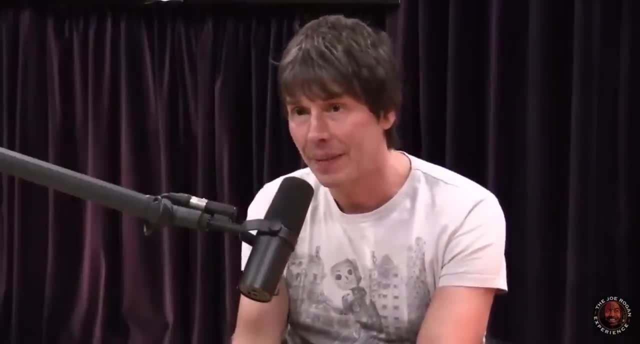 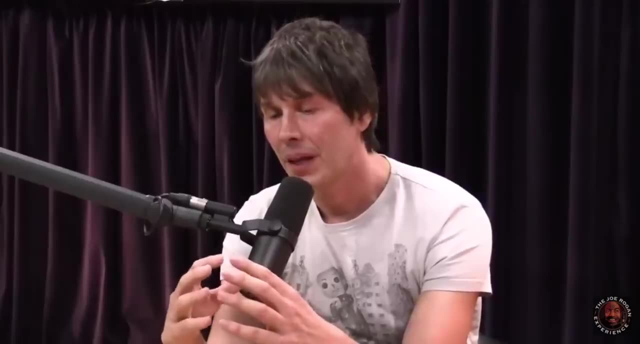 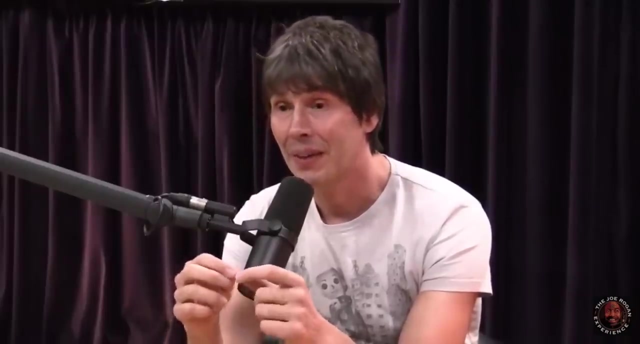 No, If something like the sun, We have a small star- It's quite small, yeah, And when it collapses, there's a sort of a pressure, a force, if you like, which is caused by the fact that electrons don't like to be very close to each other. 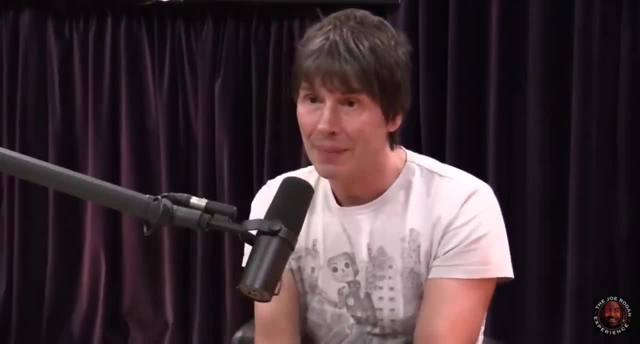 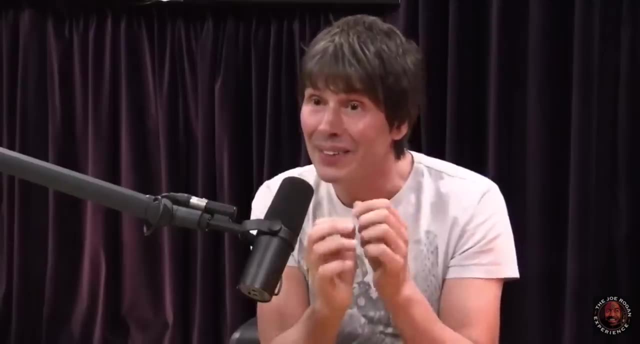 So it's called the Pauli exclusion principle. But essentially what happens is that so, as they get squashed closer and closer together, they move faster and faster to get out of each other's way, if you like Right- And that makes a force which holds them up. And so that creates what's called a white dwarf star. So you can have a blob of matter. They're about the size of the earth, but they're about the mass of the sun, And so that's for smaller stars. They end up as these white dwarf things, which are very dense objects. There's another version which is called a neutron star, which is the same thing but for neutrons, And they move faster and faster. So if it's massive enough that it overwhelms the electron, Then the electrons sort of crush into protons and turn into neutrons. And the whole thing starts again, And so a neutron star can be, you know, at least one and a half times the mass of the sun, let's say, But it can be about what? 10 miles across. So that's an incredibly dense ball of matter held up by this. The neutron's moving around. It's got a fancy name, It's called neutron degeneracy pressure. But if you go even bigger, then even that can't hold it And as far as we know then there's no known force that we know of that can hold the thing up if it's too massive. 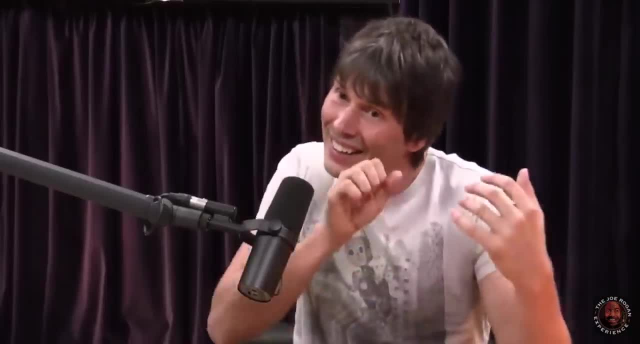 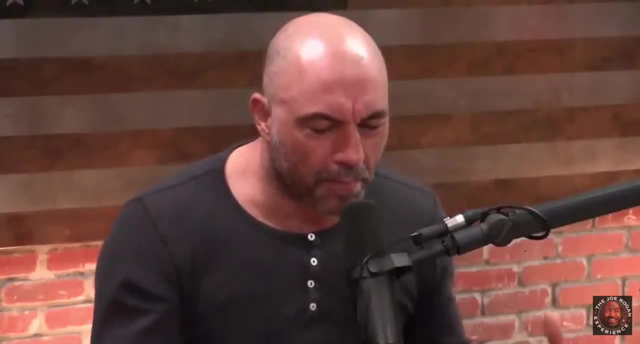 And so that's when it just almost winks out of existence, if you like. It collapses and collapses, and collapses, And that's when you get a black hole. We try to put that into perspective. The sun is a million times bigger than the earth. And this neutron star is, would you say, one and a half times the mass of the sun, but 10 miles wide. Yeah, Yeah, And there's loads of those around. They're called Pulsars, So we see those all over the place. 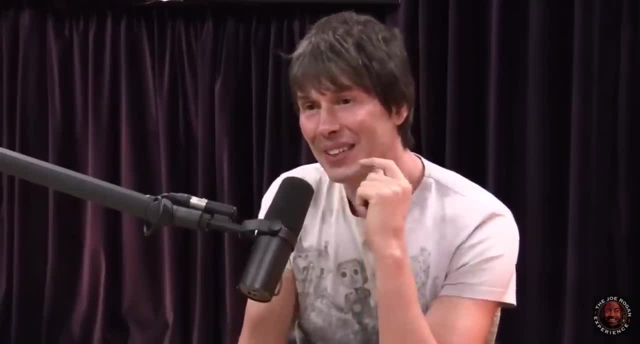 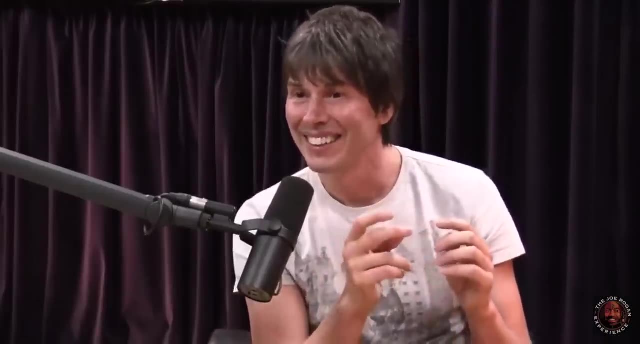 The first one that was discovered was called LGM-1 because they spin very fast, And then it was called LGM-1 because it's a very regular pulse and they thought it was little green men, So they called it, kind of jokingly, little green men one.